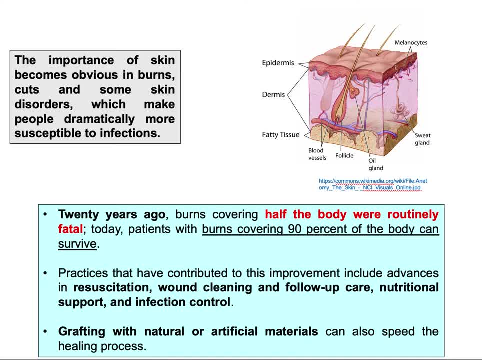 you know, problem with the skin you you're susceptible to infections and this is a big problem for anyone. and i want to draw your attention to something: if we are implanting something in the human body or implanting material inside the human body, we have to breach this. 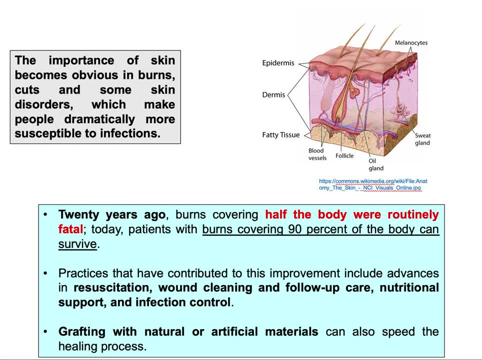 defense line. so we need to make a cut most of our materials in order to be implanted inside the body. we have to do invasive surgery in order to get the materials inside the body, like total hip and joint replacement plates and screws and all the other things. so about about the skin? so 20 years ago burns covered half of 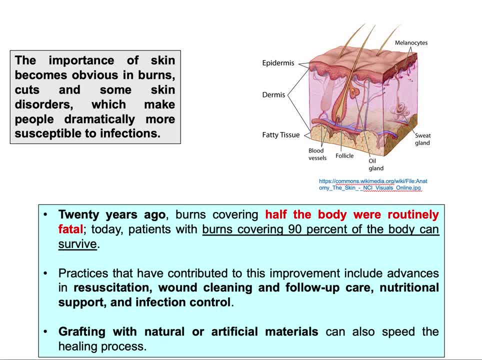 the body were were lethal, and so anyone who has burns, it's it's just lethal, they can't survive it. but nowadays we we have a lot of technologies and we have improved our interventions so that even someone with 90 percent of their body burned, we they can survive. they have a good chance of 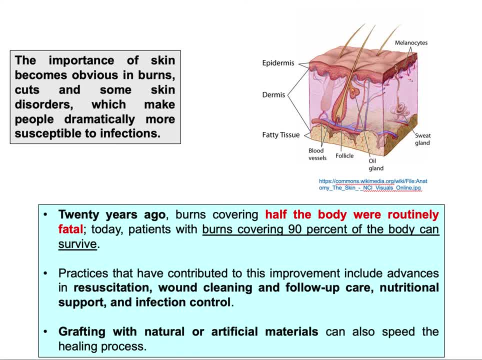 surviving, and there are a lot of people who are suffering from burns and they have a good chance of surviving, and there are a lot of good reasons, uh, why that's possible, and so the practices have been contributed. this involvement improvement included race citations, wound cleaning, follow-up. 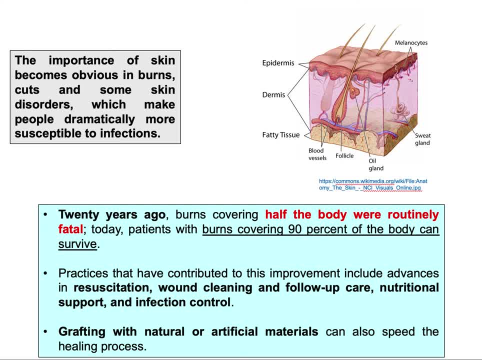 care, nutritional support and infection, called infection control. we did a lot of good work so far in protecting the body in case of damage of barrier, of the of the barriers. also, we have a big field of research and there's huge marketing improvement discussion about if, yes, uh, looking to start giving the most Crzy muslim member Youre'. 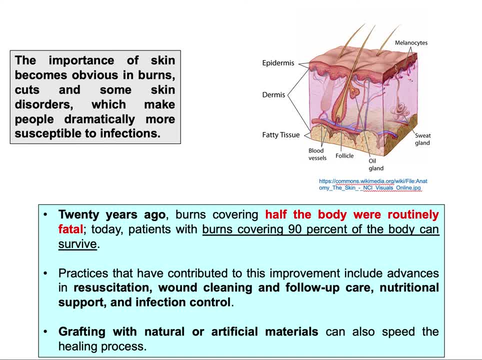 I have teeth by cr Gates Co, certain the, especially if they're seeded with endothelial cells that can create the skin layer that we wanted to be there. So again, skin is very important and we're going to talk more and more about how the skin 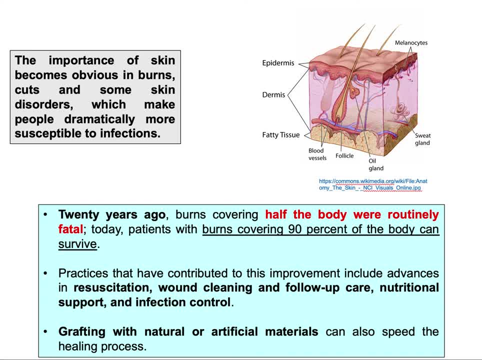 is playing a crucial role in the immune response, which is actually a determinant of the success of our material inside the body. So this is a schematic of the skin, different skin layers and components, and there's a lot of things happening inside here that can affect.